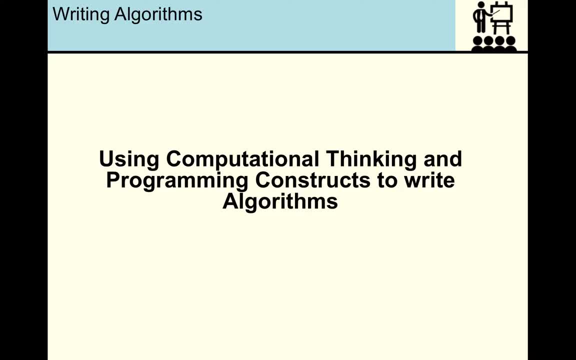 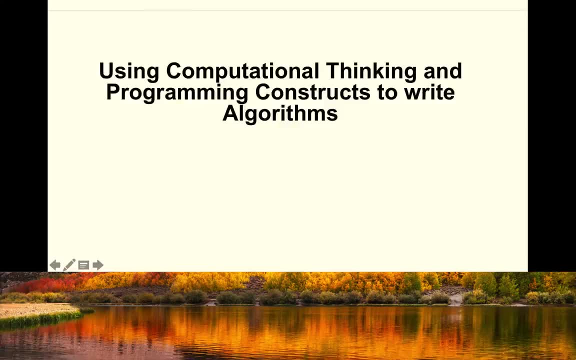 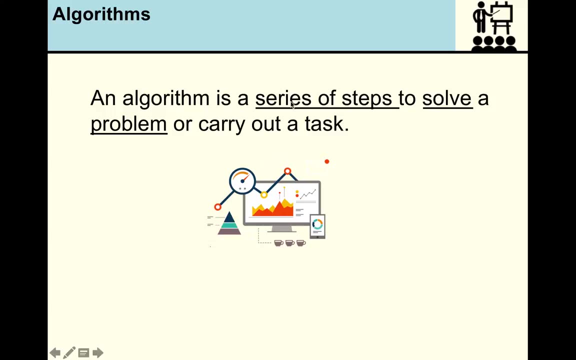 In this video, we're going to look about how we can use computational thinking and programming constructs to write algorithms. We're going to be combining our knowledge of computational thinking and programming constructs to write algorithms. Now, an algorithm is a series of steps to solve a problem or carry out a task. It's a series of steps. Now, it's important for you to remember that. 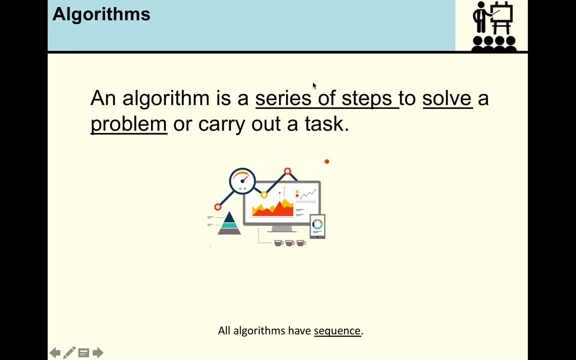 all algorithms have sequence, and sequence is the same as a series of steps. Sequence is a series of steps. All our algorithms have sequence. They're all written as a series of steps. Now we've talked about solving a problem. What is problem solving? Now we encounter? 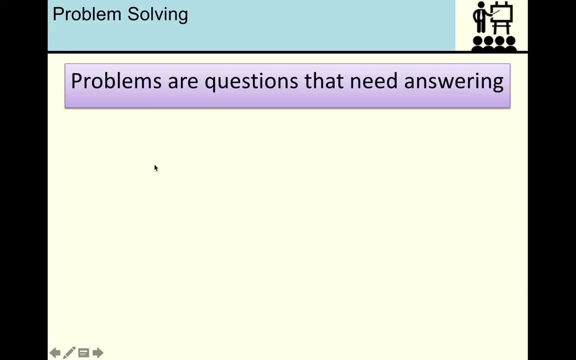 problem solving in everyday life, and problems are questions that need answering. Problems are just questions that need answering, and we have questions like how do I get to that location, Or what video should I watch next on Netflix. Those are all problems that algorithms have been written to find solutions to. 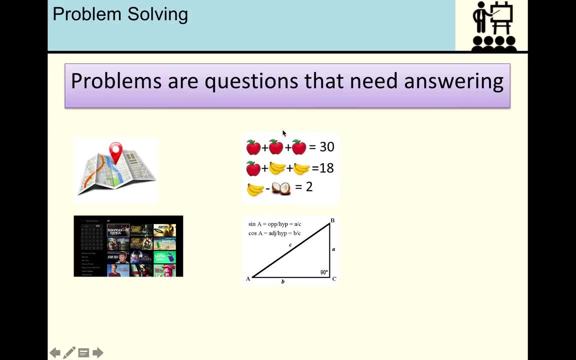 In maths you write algorithms. In maths you answer these problems using algorithms. You answer the problem of how do you work out the angles of a triangle. These are all problems, And in computer science you have problems like how am I going to sort this information? 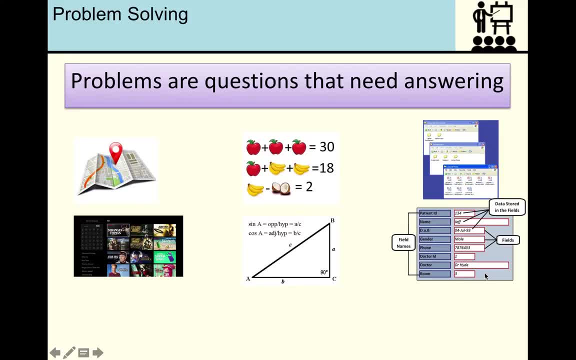 into order, or how am I going to store information in memory And remember? an algorithm is a series of steps to solve a problem or carry out a task. Now, in your exams, your problems are the questions that need answering. What is a computer system? 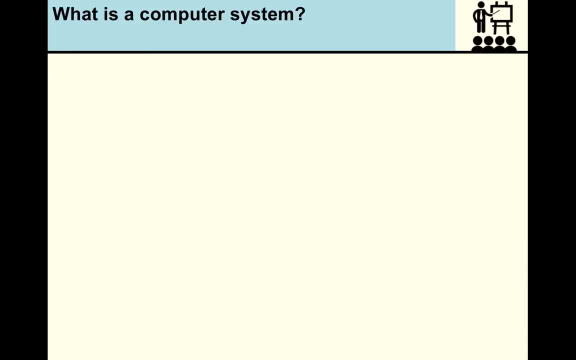 Now, this is the most basic of computing constructs. A computer system takes inputs, it processes them and it produces outputs. Inputs are like electronic signals, like a mouse click or a keyboard press, The process. when we process information, we're actually encoding and executing instructions. 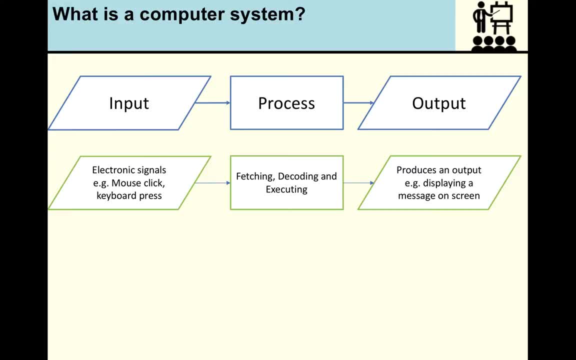 And finally, our output is. where we can, We can display something or output something. So right now my input is the microphone, The process is converting my voice from analog to digital And the output will be playing that sound through the speakers. 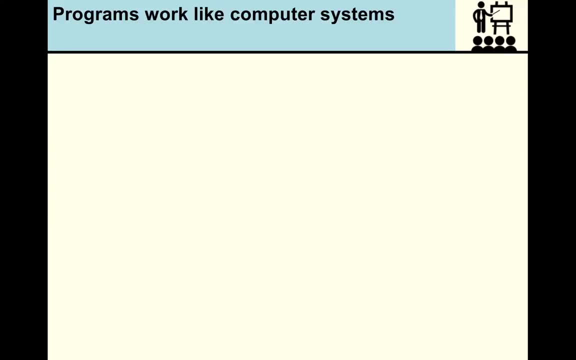 Now why is this relevant? Because, just like a computer system, programs work the same way. Programs take inputs, they process them and they produce outputs. In our programs, our inputs are data entered by the user or information entered by the user. 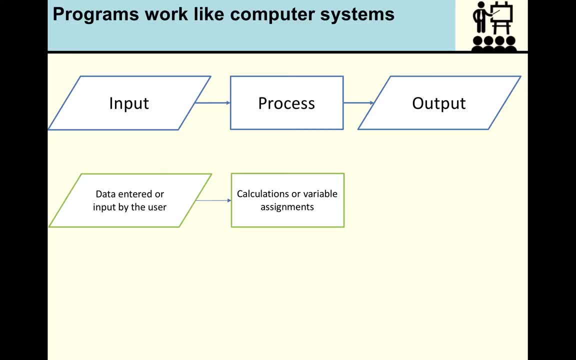 Right. So our processes are calculations or assignments to variables, and our outputs are displaying a message or the result or values to the user on the screen. So remember that our programs take inputs, they process them and they produce outputs as well. 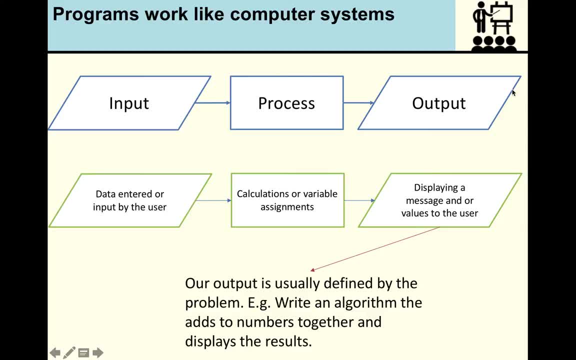 And we usually know our output if we work backwards, because our output is usually defined in the problem. So when we write an algorithm that adds two numbers together and display the results, our output is the results. Our process is adding those two numbers together. 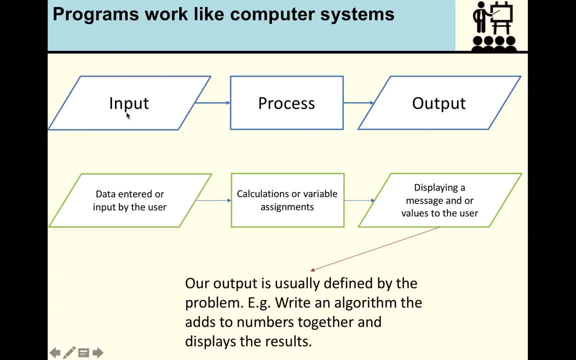 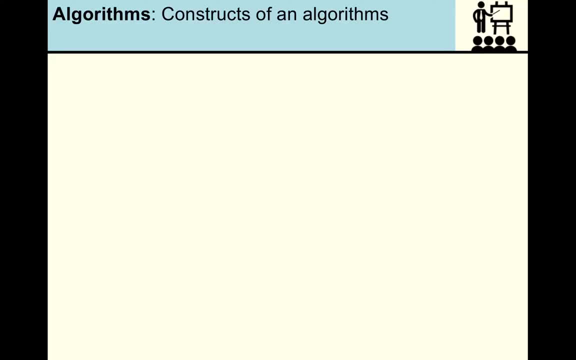 And we can even think further back and say: what do our inputs need to be? Well, those inputs need to be two numbers. So what are the constructs of an algorithm? Or what are the constructs of a programming language? Well, see if you can guess them from these images. 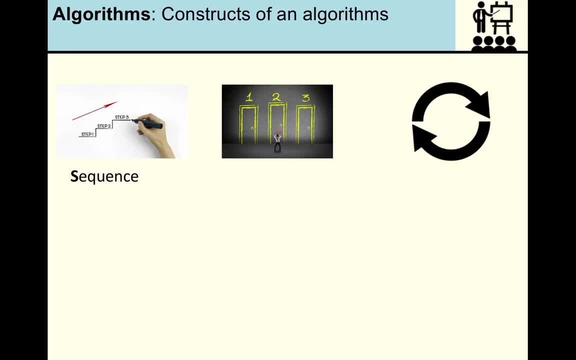 Well, our first construct we've already mentioned and that is sequence, And all algorithms have them. They are a series of steps And they are, They are always sequential. Our programs start at the top and they work their way through. 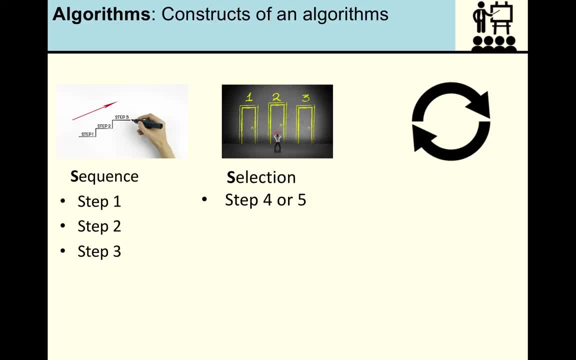 Now the second one is selection, And that's when our program has to decide whether it goes to step four or step five. It has to make a decision. Is it door number one, door number two, door number three? And we make decisions, and those are in selection. 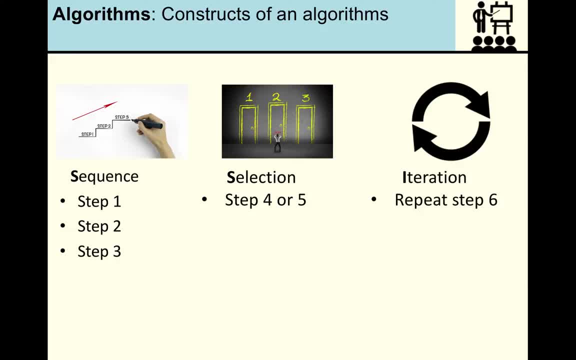 And finally we have iteration, where we repeat a step. We repeat a step, Or we might repeat several steps, and that's iteration. So in programming we have sequence, Sometimes we have selection And sometimes we have iteration, But we always have sequence. 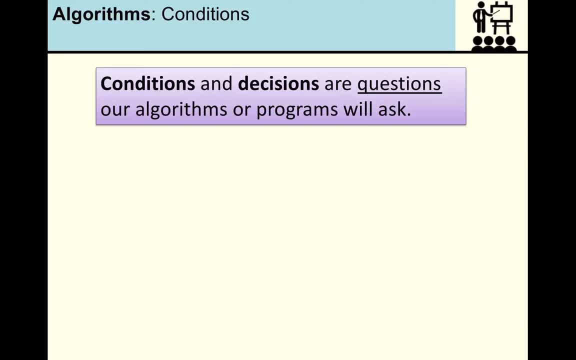 And we also have conditions. Now, conditions and decisions are questions our algorithms or programs will ask. So if our computer is going to make a decision, there's usually going to be a question in there: Which decision, which route, which path do I take? 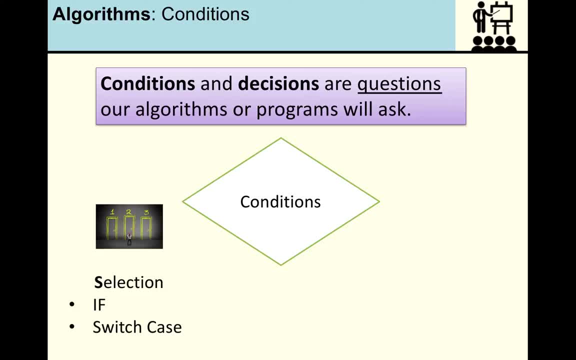 And our conditions are represented with a diamond, And those are usually selections. So if this is true, I'll go through. I'll go through. I'll go through number one, Else I'll go through number three, Or we can use switch case statements. 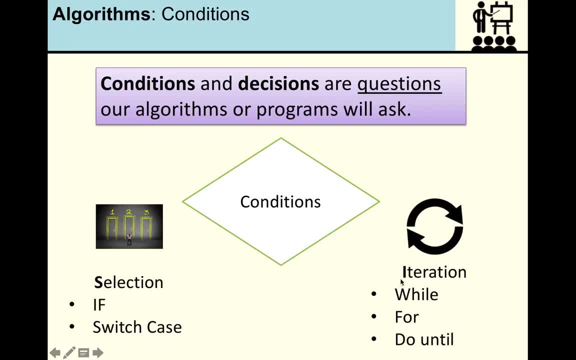 And we also have conditions for loops. So, while the user gets their password wrong, allow them to input it. Or, for three attempts, let the user input their password And our question there would be: has the user entered it three times? 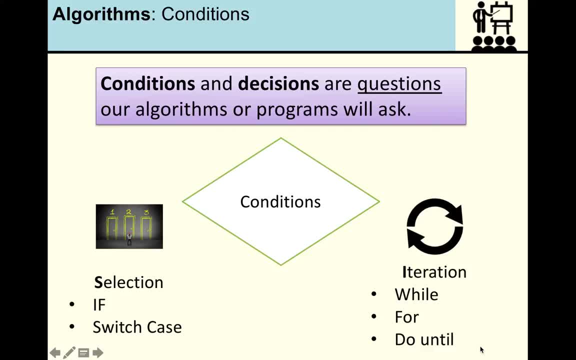 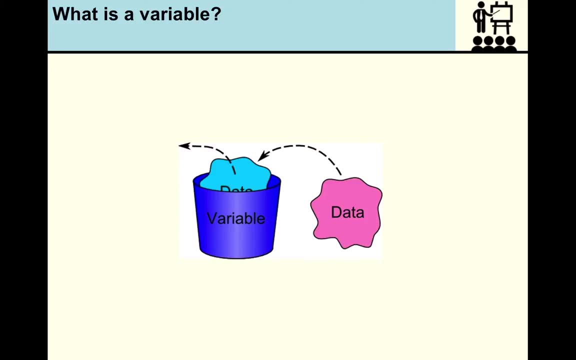 Or do until We do something, until a condition is met. Allow the user to enter their password, until they enter the correct password. So conditions and decisions. We also have conditions and decisions in our problems. And finally, we need to remember what a variable is in our programming constructs. 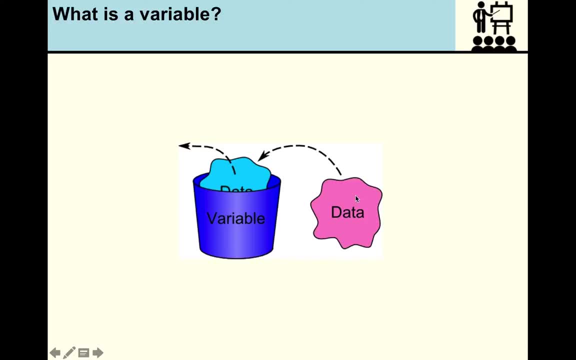 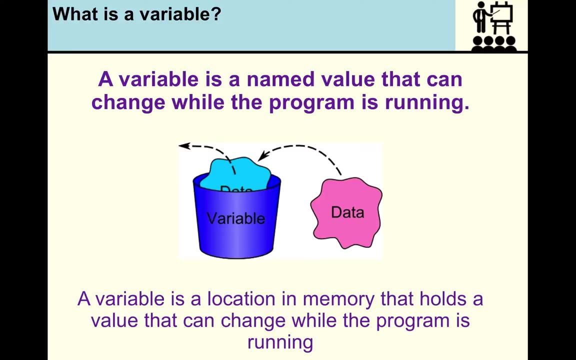 So a variable? because when we program, we're programming with data that can change, And a variable is a named value that can change while programming is running. While a programming is running, A variable is a named value that can change while the program is running. 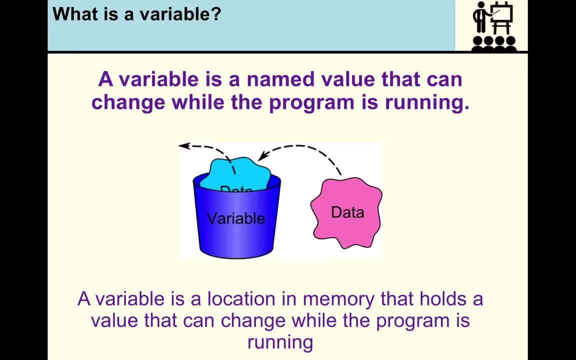 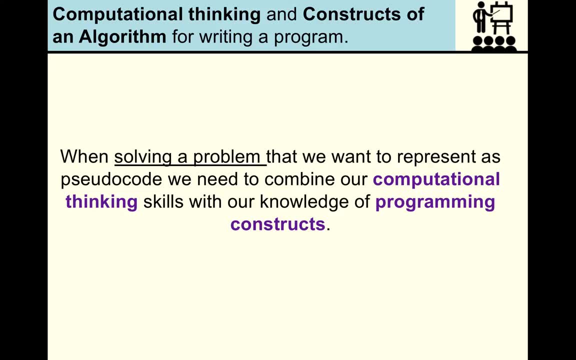 And for a higher level. a variable is actually a location in memory that can change And it holds a value while the program is running. Now we want to tie together our constructs of an algorithm with computational thinking And, if you remember, computational thinking is all about solving problems. 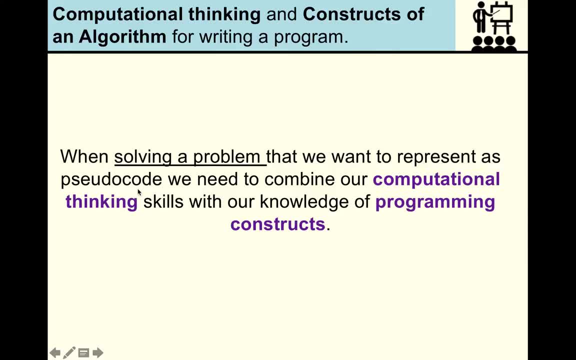 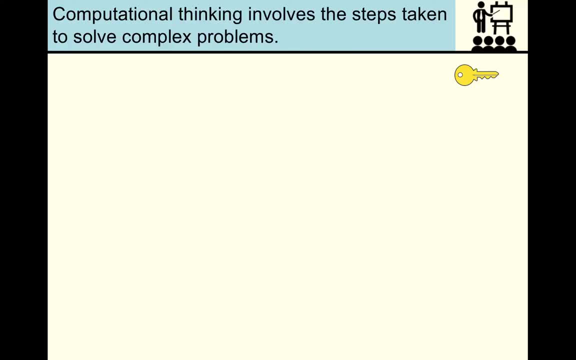 And when solving a problem that we need to present a pseudocode or an algorithm, we need to combine our computational thinking skills with our programming constructs. So computational thinking Involves the steps taken to solve a problem, The steps taken, The steps taken. 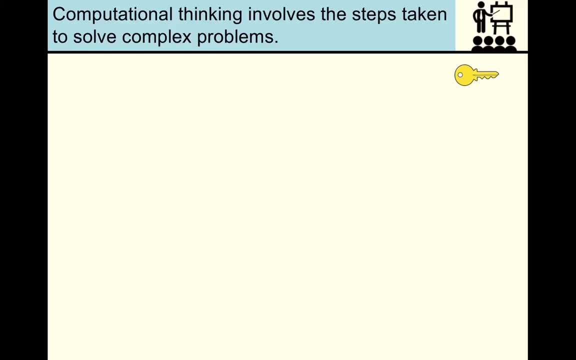 So computational thinking is how we figure out what those steps are, And the first step in computational thinking is decomposition. Just like in biology, decomposition- When something decomposes, it breaks down, And for us to work out our problems, we need to break them down into smaller sub-problems that are easier to solve. 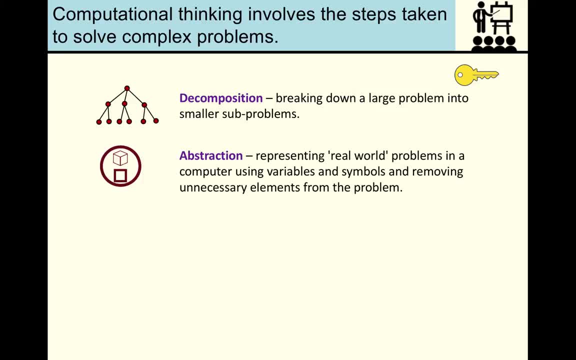 Abstraction is where we represent real-world problems like: how do I represent a picture of the world as a map? We need to represent real-world problems in computing terms And we need to use variables and symbols removing unnecessary elements from the problem. 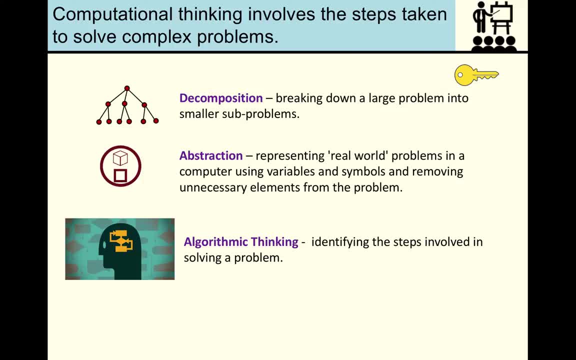 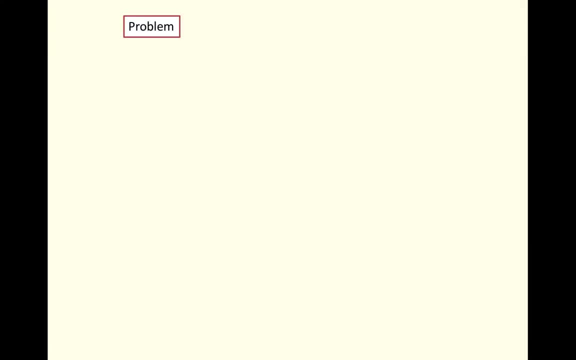 And finally we have algorithmic thinking, where we identify the steps involved in solving a problem. So I'm going to demonstrate now how we apply computational thinking to solving a problem. Remember, our problem is a computer, Our problem is a question. 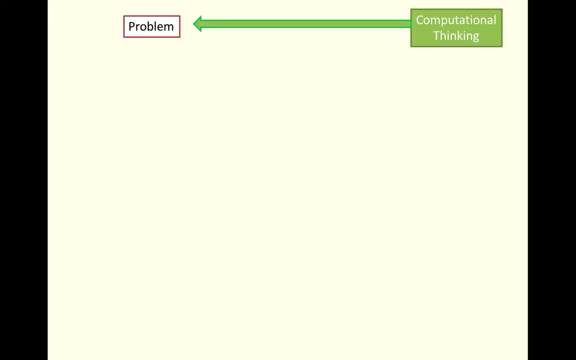 Our problem is a question that needs to be answered And we need to apply computational thinking to solve that problem. So the first step that we do is we decompose our problem. We decompose our problem and we decompose it into inputs, processes and outputs. 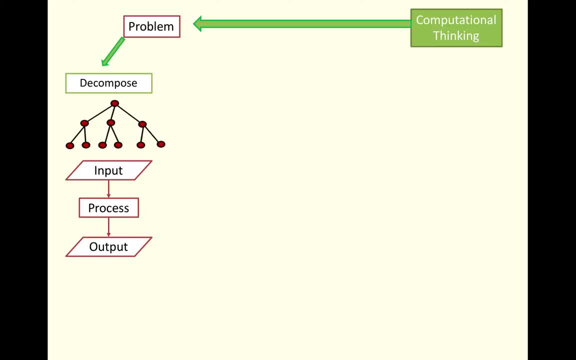 Because those are the constructs of a program. They take inputs, they process them into outputs. So we need to look at our question, We need to look at our problem. We need to think: what are the outputs? What are we trying to achieve? 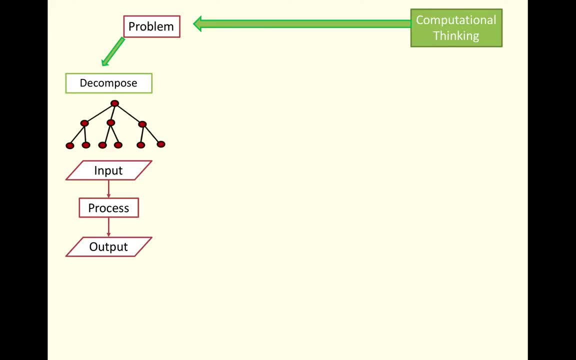 What calculations need to happen and what do we need to input for this to happen? So we need to decompose our problem into inputs, processes and outputs. We then need to use abstraction to figure out what our variable's going to be. 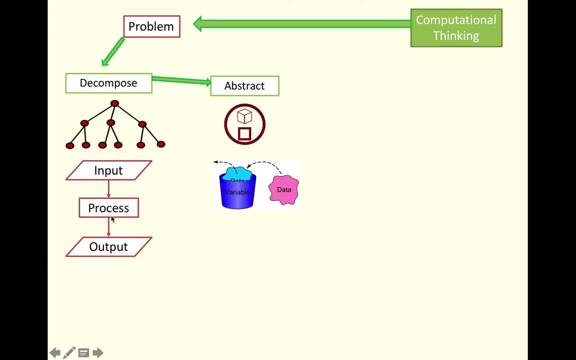 Where are we going to hold all our input values? Are we're going to store the results of the calculations? where we're going to store them in variables? And our outputs, our outputs? Do those need to be held in variables as well? 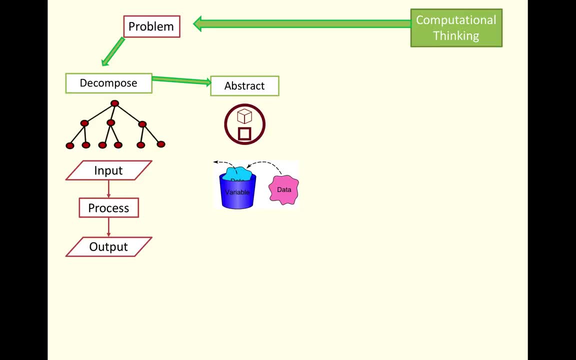 OK, Once we've decomposed our problem, once we've broken it down into smaller sub-problems- like what are our inputs, what are our processes and outputs- and we've abstracted the relevant information out of our problem, we're also going to check what are our conditions. 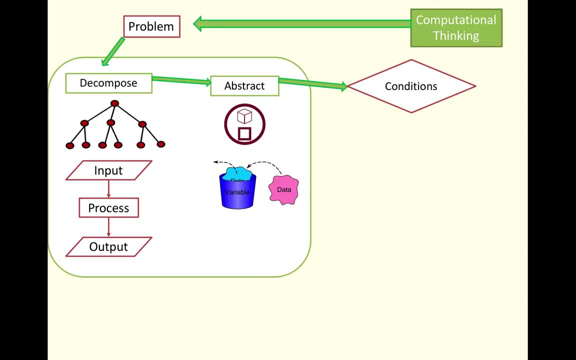 So all programs have sequence, but they don't always have conditions. But as they get more complex, there'll usually be some form of selection, some kind of decision or path that we need to check. if we're going to take- And we're also going to have iteration, we're going to have iteration, we're going to have iteration, we're going to have iteration. 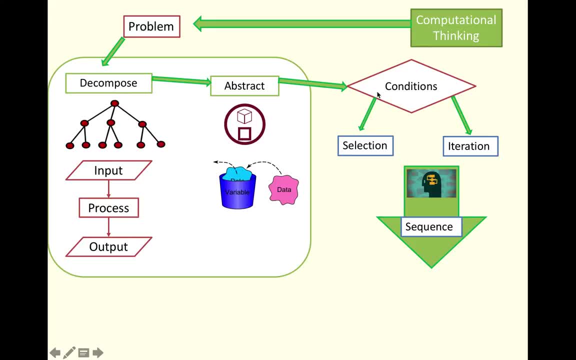 That's where we repeat a step And when we've checked for all our conditions and questions and we've got all our variables and we know our inputs, our processes and outputs, we need to use algorithmic thinking to put this into sequence. 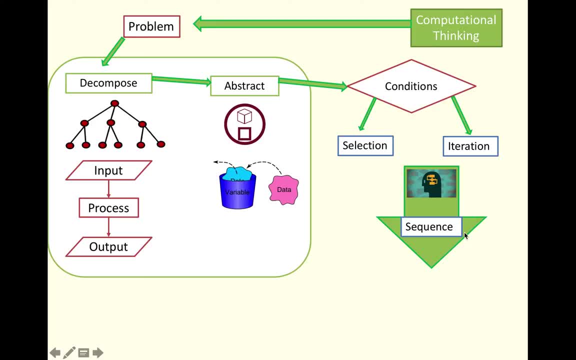 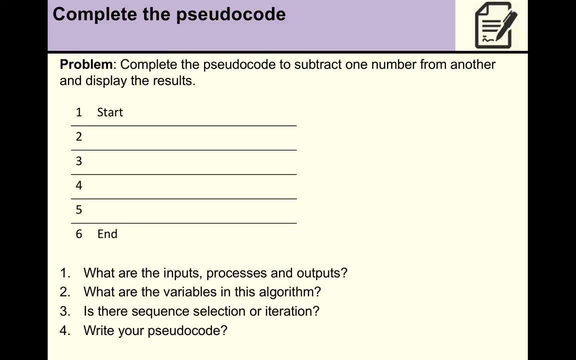 We need to use algorithmic thinking to put this into sequence And we finally produce an algorithm which is a series of steps- Steps to solve a problem or carry out a task. So I'm going to go over a quick example of a very simple problem where we need to subtract one number. 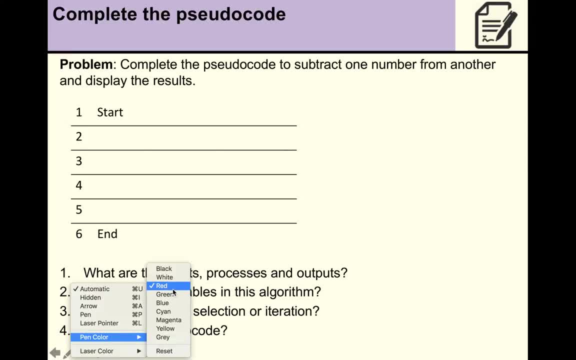 We need to subtract one number from another number and display the results. Now, whenever you approach an algorithm question, I want you to ask these first three questions: What are the inputs, processes and outputs? What are the variables in this algorithm, And is there sequence selection or iteration? 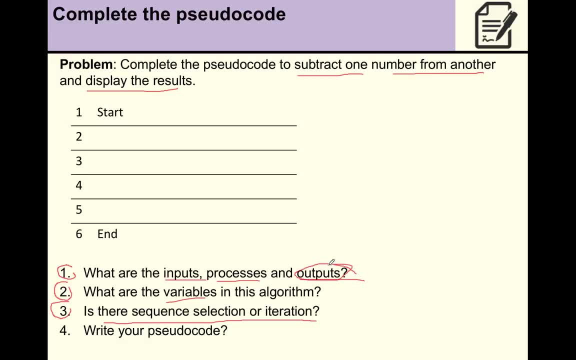 So the inputs, processes and outputs. let's start from the back. Our outputs are. we're going to display the results, Because display is a trigger word for output And we need to display the results. In order for me to display the results, I need to perform a process. 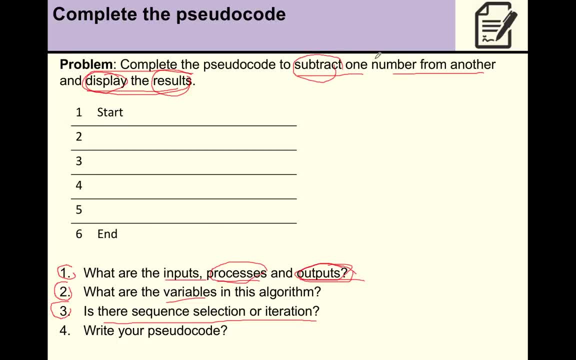 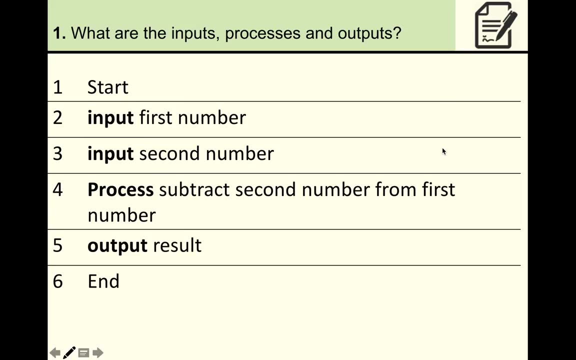 And that process is subtracting one number from another, And in order for me to subtract one number from another, I need to have those numbers. So those numbers are going to be input into my program. I need to input those into my program. So what are the inputs, processes and outputs? 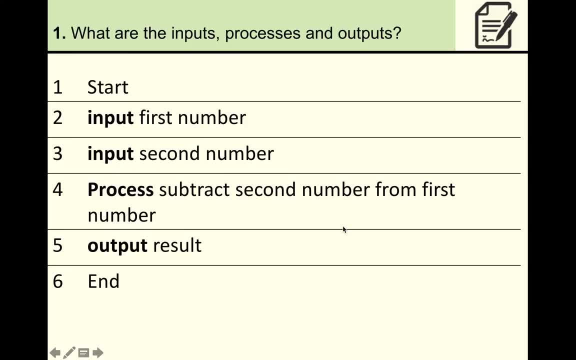 Well, I need to input my first number, I need to input my second number, I need to process them- and that's a calculation subtracting the second number from the first number- And finally, I need to output the results. Now, what are the? 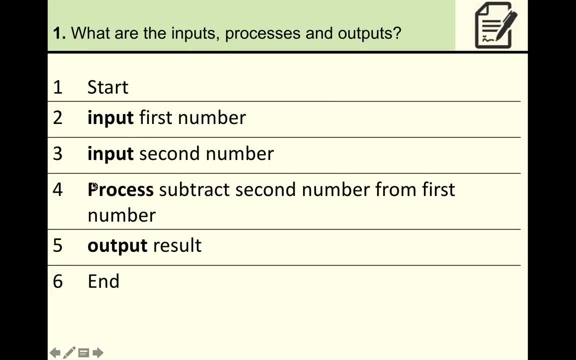 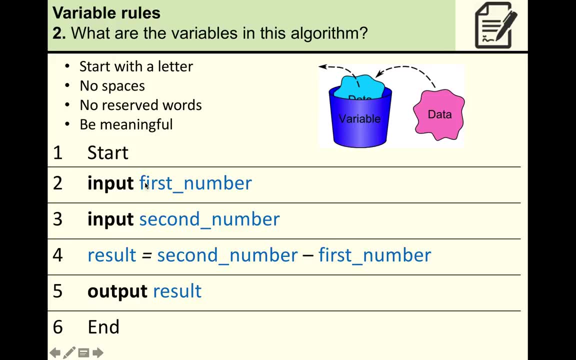 variables in this algorithm. So I've got these inputs, I've got a process, I've got an output, but I need somewhere to store these numbers. So my input is my first number and that's my variable name And it follows the rules of how we name variables. Now, before it was quite simple. 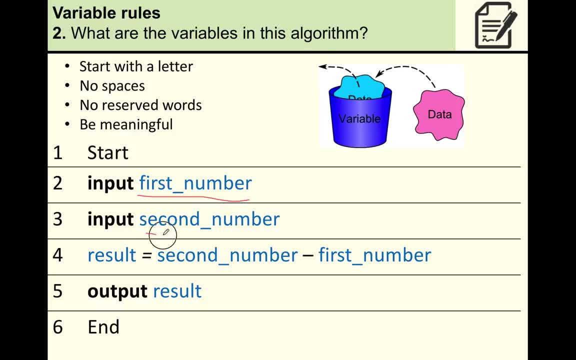 because I know that if I'm inputting something, I need a variable to hold it. If I'm inputting something, I need a variable to hold the value. But when I perform a calculation, when I perform a process, I need to remember that I need 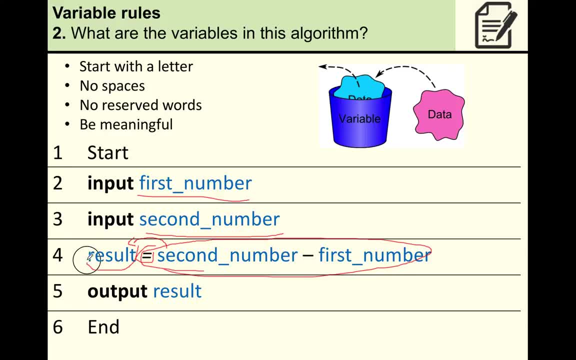 to assess the radiative values that are performing, that are affecting. that shall be a variable to hold the value. But when I perform that I need to assess the that value. I need to assign the results to a variable. so I'm going to call my variable result and then I can display the value that's stored inside result. 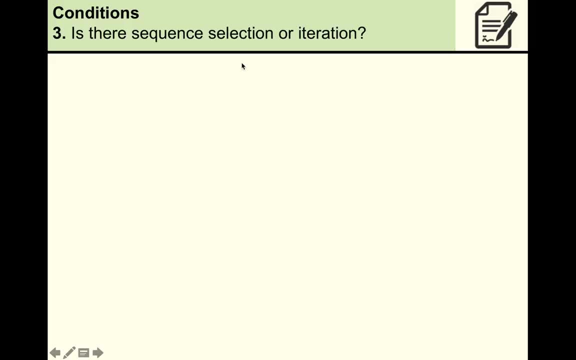 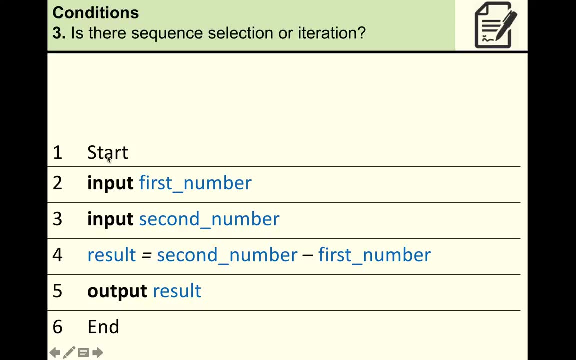 Now the last question was: is there sequence, selection or iteration? Well, all programs have sequence. All programs have sequence and we can see that sequence here, because I need to start from start. I then need to input my two numbers before I can process them and I need to process it before I can produce my 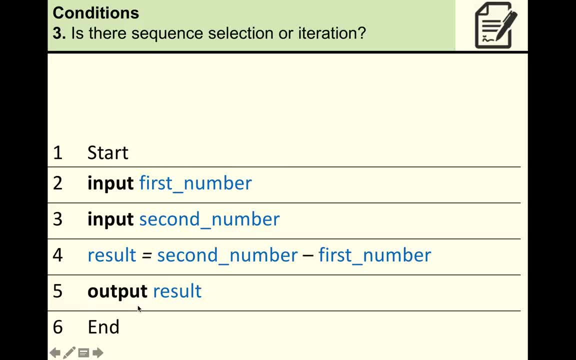 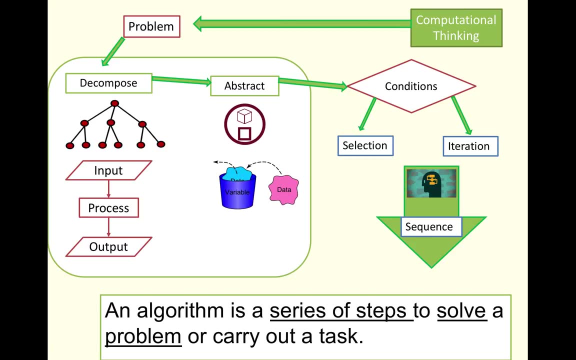 result. So all programs have sequence. In this case, there are no questions or decisions being asked, I don't have any selection and there are no steps being repeated, so I don't have iteration. Remember, in order for us to solve a problem, we need to apply computational thinking to that problem and we need to